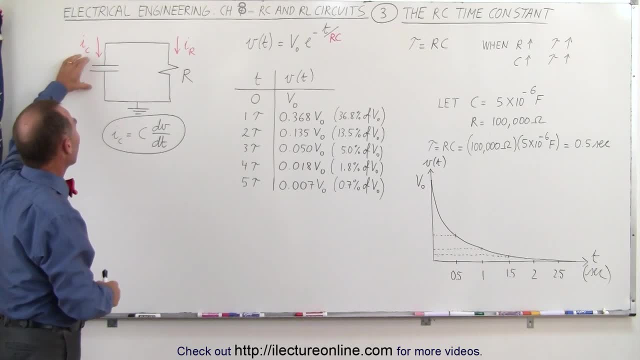 will charge. In this case, we assume that the capacitor had an initial charge on it called Q, sub naught, and over time the charge will simply leak off from one side, go to the resistor, go to the other side until the capacitor is no longer charged. 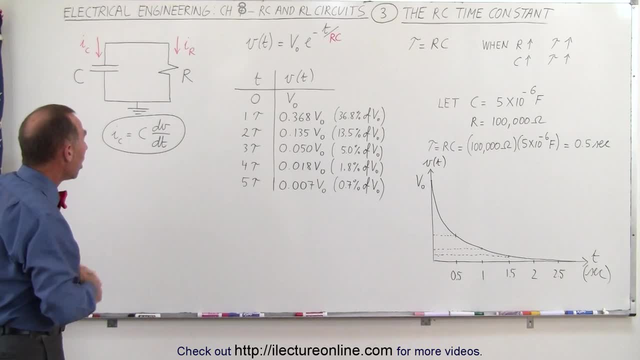 With other words, until the charge on both sides of the capacitor is equal. How long will that take? Well, that depends on the time constant. Now imagine if you had a much bigger capacitor, a capacitor that could hold a lot more charge. So, for the same initial voltage, the capacitor. 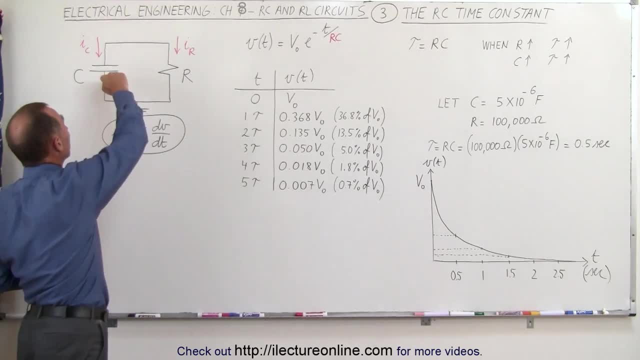 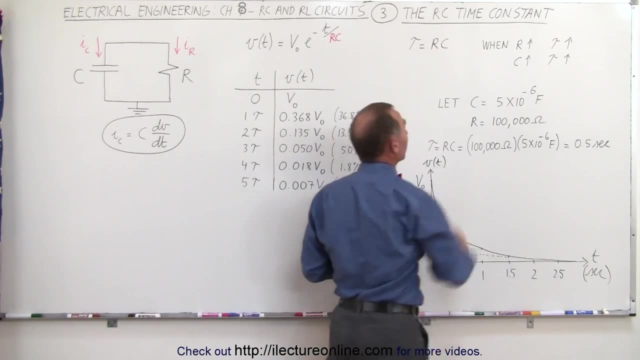 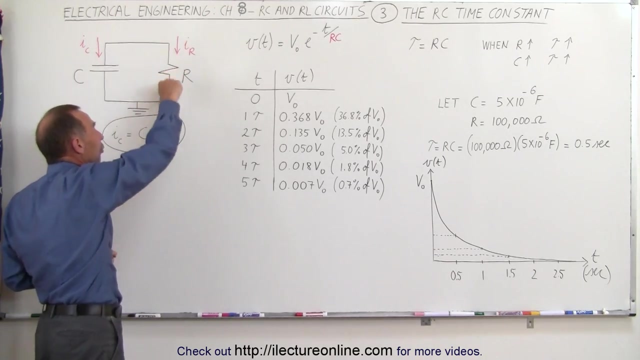 would then contain a lot more charge and therefore it would take a lot longer for the capacitor to discharge. which means, therefore, that if the capacitance is larger, the time constant would be larger. Well, if we had a larger resistor, it would not allow as much current to flow through. 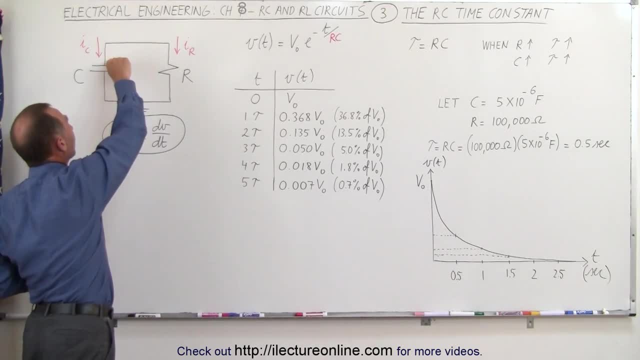 the circuit, which means it would take longer for the charge from one side to run through the resistor or to flow through the resistor. The charge doesn't really run, it flows through the resistor to the other side. Again, a larger resistor means smaller current, which means 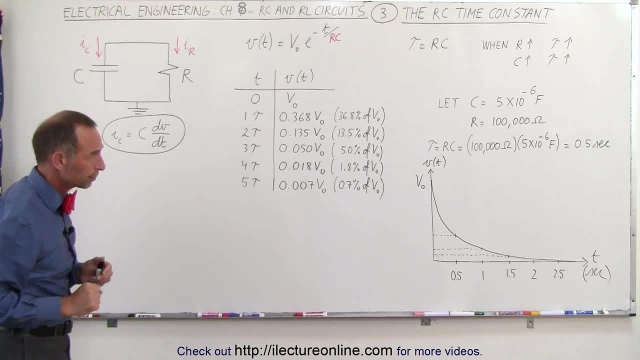 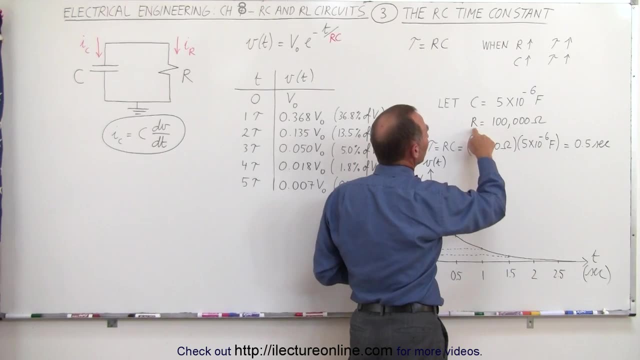 it would take longer for the capacitor to discharge. As an example, let's say that we had a capacitance of 5 microamps, 5 microfarads, And we had a resistance of 100,000 ohms. If we multiply those together, 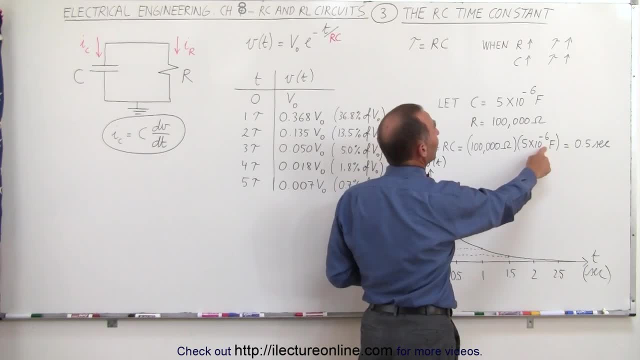 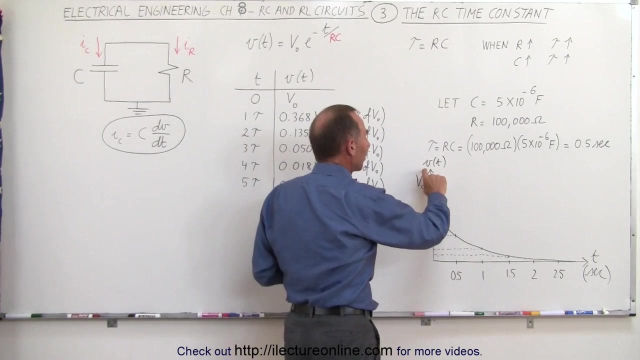 R times C, 100,000 times 5 times 10 to the minus 6, gives us a half a second. In the next video I'll show you where the units of second comes from. multiplying ohms times, farads. Now here we have a graphical representation of the voltage across the capacitor as a function. 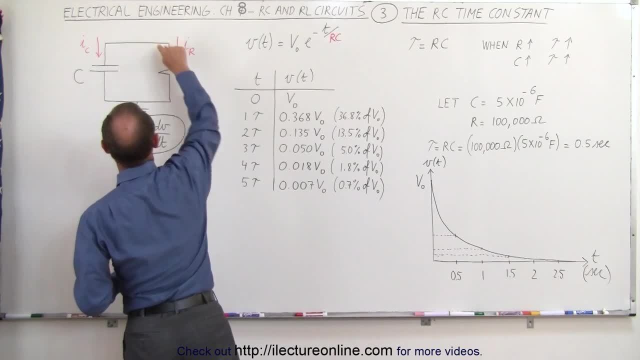 of time. Notice as charge leaks off one side and you can see that the voltage across the capacitor is a function of time. Notice as charge leaks off one side and you can see that the voltage across the capacitor is a function of time. Notice as the charge. 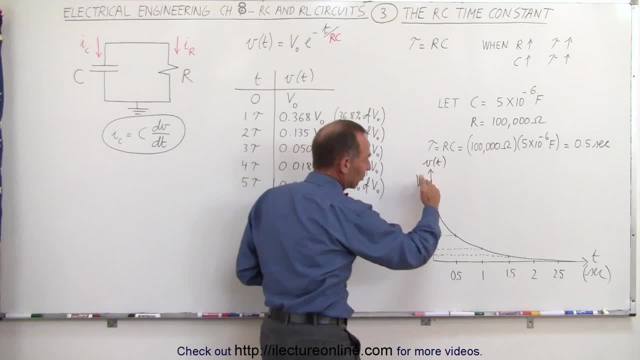 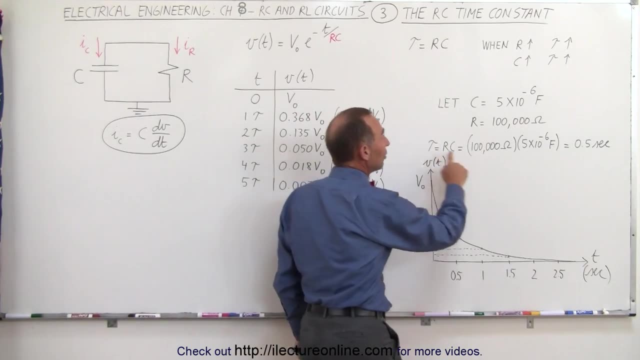 goes one side and the voltage across the capacitor goes to the other side of the capacitor. until the capacitor is discharged, the voltage across the capacitor will decrease like this exponential decay curve. Notice that if the time constant is equal to a half second after, 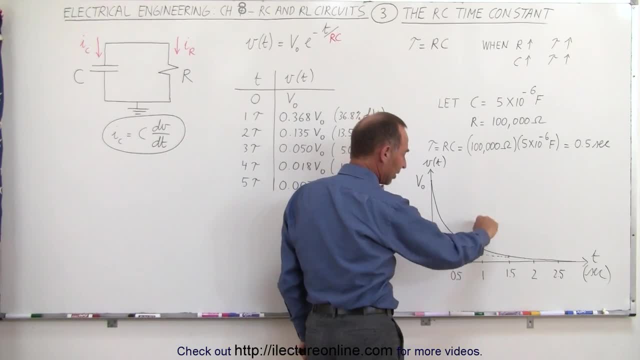 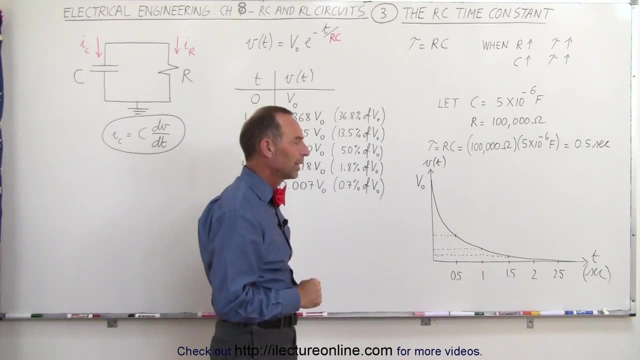 a half second, the voltage will have dropped to this amount. after one second it will continue to drop, and so forth, and eventually, as time reaches infinity, then of course the voltage will go to zero. Now that's not really a practical concept in electronics, because 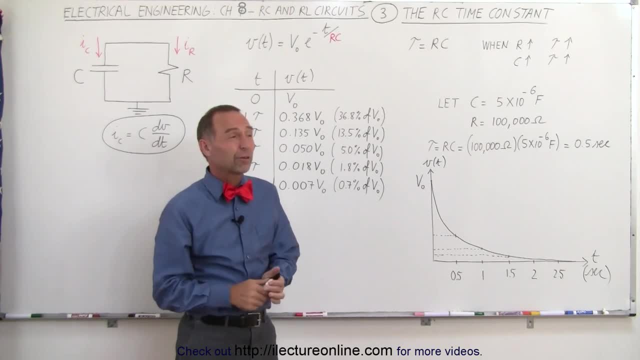 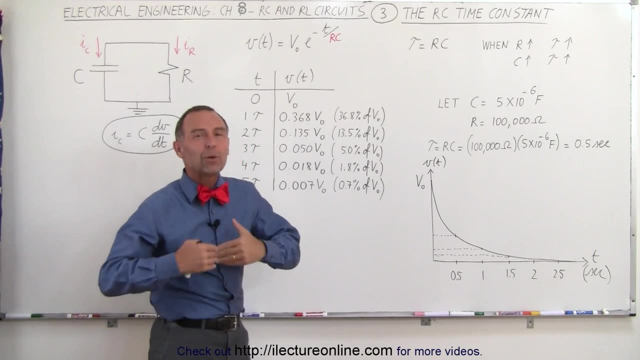 If we have to wait until time is infinity before there's no more voltage across the capacitor, that doesn't make a lot of sense. After a while, the voltage will be so small across the capacitor that we can consider it zero in all practical purposes. 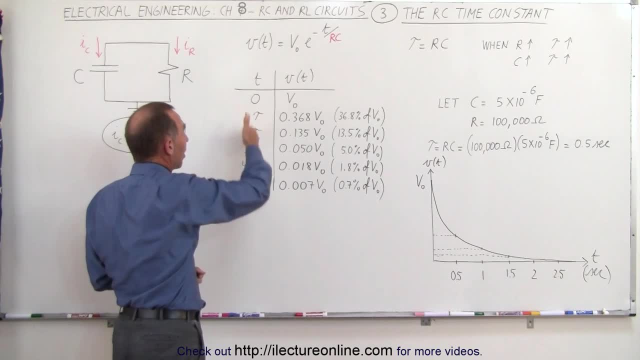 To give you an example here. numerically let's say that here we have a column that represents the time elapsed and the voltage remaining on the capacitor. When time is equal to zero it has the full voltage across capacitor V sub naught, But after one time constant. 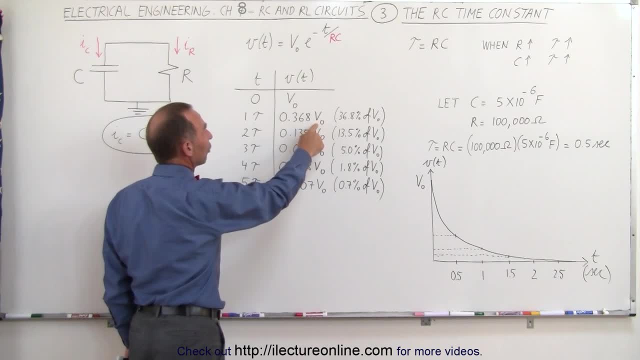 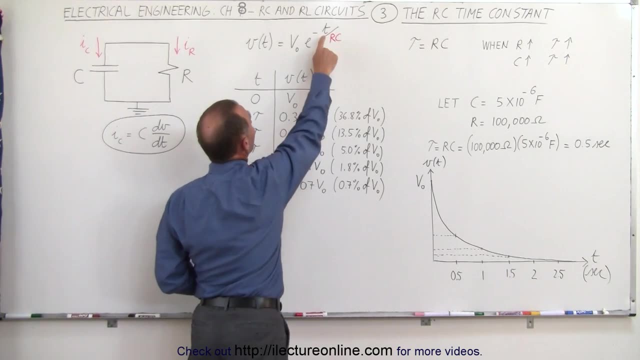 the voltage has decreased to 0.368 times the initial voltage, or 36.8% of the initial voltage. How do we figure that out? All we have to do is plug in one tau or one RC in for time. we get e to the minus one. e to the minus one is 0.368. 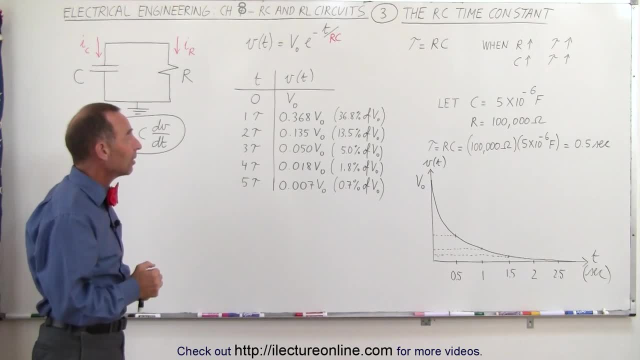 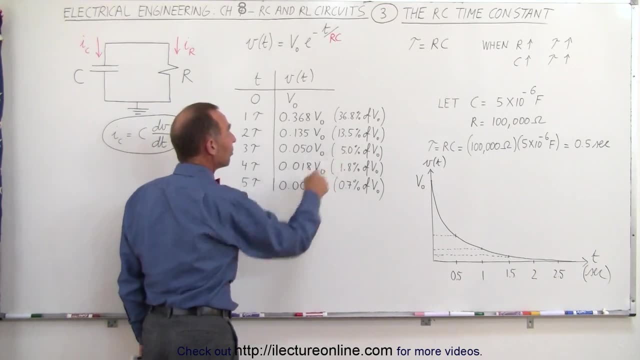 and that's how we get the voltage across the capacitor. after one time constant, After two time constant, it's dropped to 13.5%. After three time constant, it's dropped to 13.5%. After four it has dropped to 1.8% of the initial value. 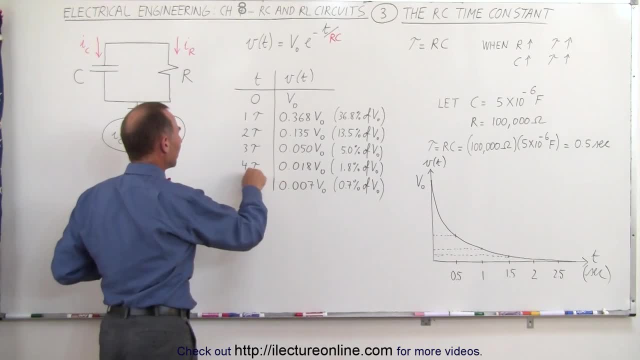 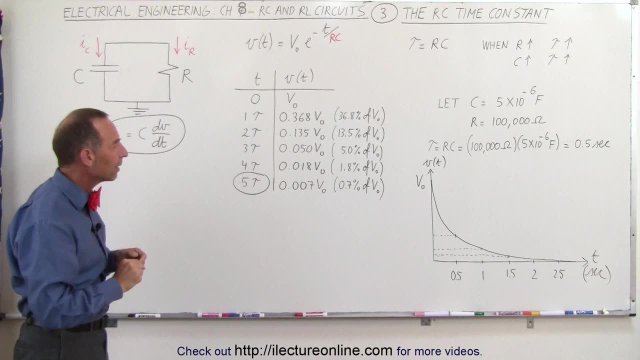 And finally, after five time constants, the voltage across capacitor has dropped to less than 1% of its initial value, the initial value of V sub naught. And so therefore we typically say in electronics that after five time constants, the voltage across capacitor is essentially gone to zero. 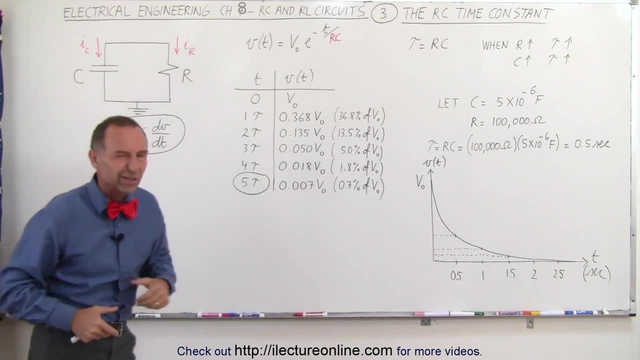 because we know at that point it's less than 1% of its initial value And in all practical purposes that would be considered close to zero- close enough to be considered zero or the capacitor is fully discharged. So that's why the concept of five time constants. 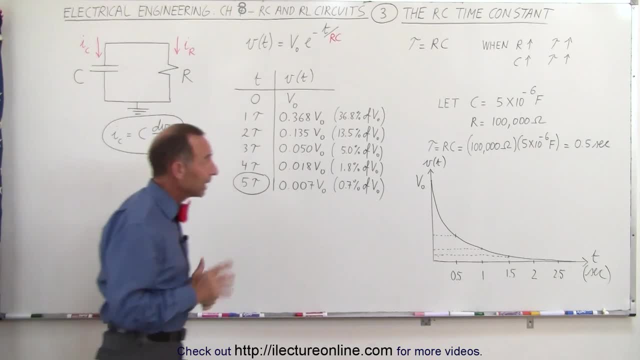 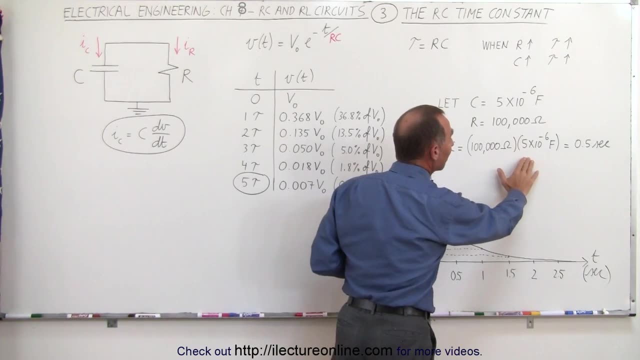 is important. So in this case, in this particular circuit, if the capacitor was five microfarads and the resistance was 100,000 ohms, it would take five time constants, or five times a half second, which is two and a half seconds.